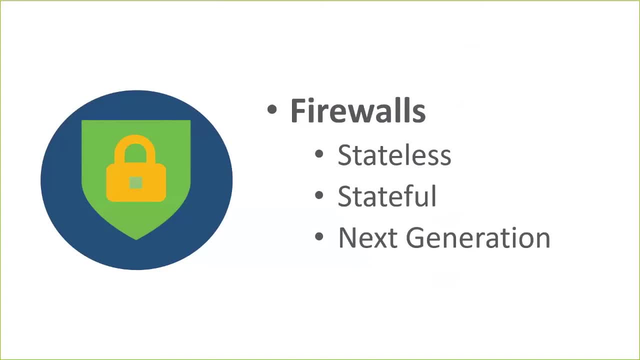 security appliance would not natively have the ability to look at which URL you're actually going to out on the Internet. But a next-generation firewall could not only know that, but it could also know what application protocols you're actually using to get to that resource. 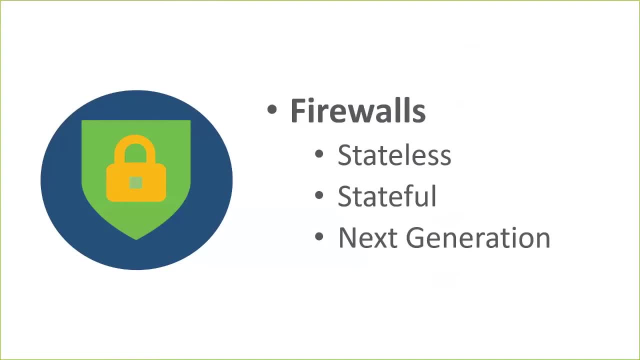 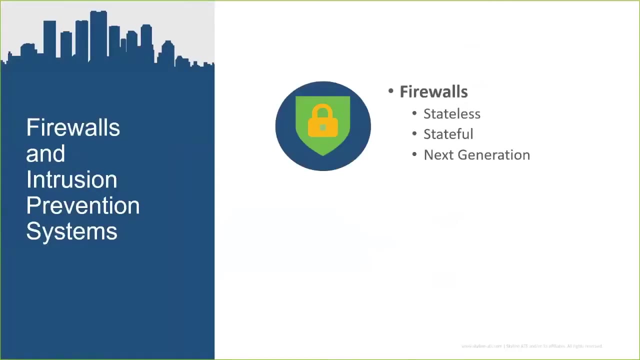 out on the Internet and then manage that effectively from an application visibility, malware, malware inspection, file inspection perspective. So next-generation firewalls combine together many of the features related to securing our traffic flows in and out of the network: Intrusion prevention systems, which are a little bit different than firewalls but can also be. 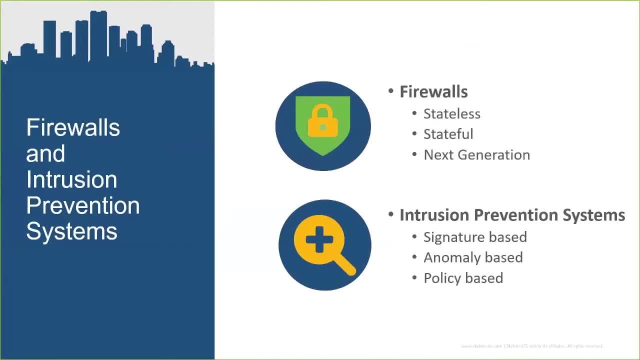 incorporated into a firewall. So, for example, you can actually have a firewall that has an IPS subsystem built into it, provide a deeper analysis of traffic flow And it's important to note that they come in three basic form factors or three basic mechanisms to actually inspect the traffic. So signature-based is where we compare traffic. 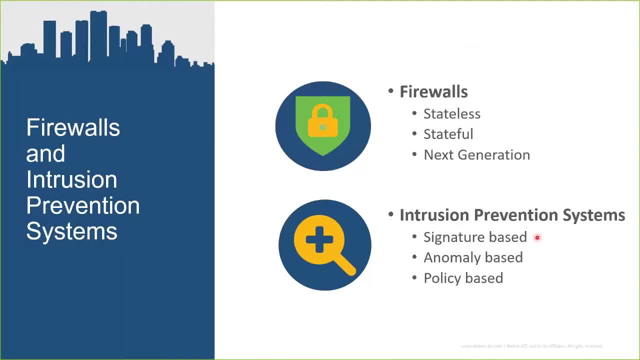 to a database of known attack patterns, So this is also sometimes referred to as rule-based or pattern-based matching. Anomaly-based is where we basically build out a statistical model of what normal traffic looks like And then, when we have, anomalies occur inside of our network which are captured by sensors. 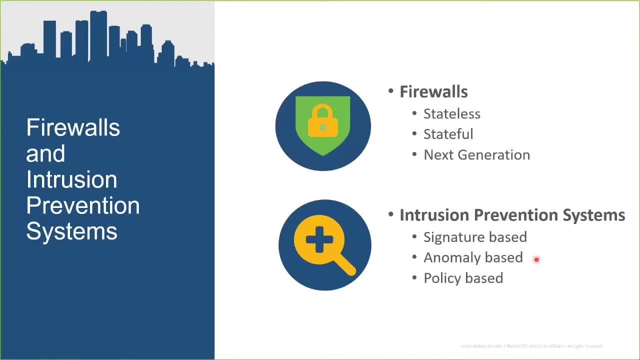 we then throw up alarms and basically say, hey, we might have a problem out here. And then policy-based is where we basically take effectively our security document and we translate that into a series of policies that we want our IPS systems to effectively evaluate and 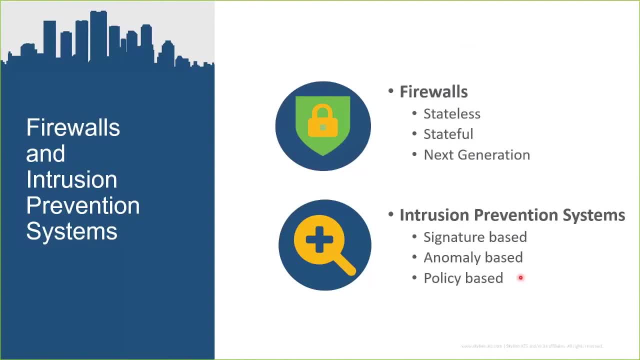 in terms of traffic flows in and out of the network. So now, as I said, firewalls and IPS systems can actually be combined in a single appliance. In fact, that's what a next-generation firewall is. excuse me, is it's effectively a marriage? 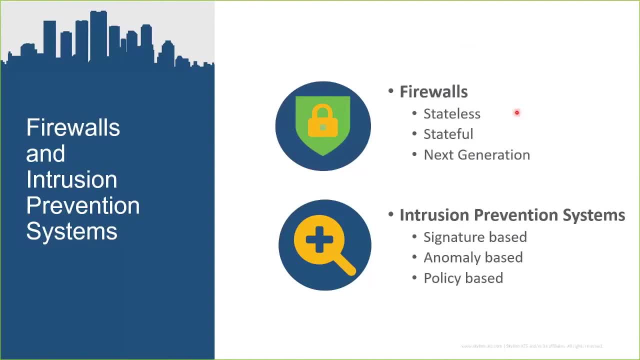 of stateful firewall connection or unit events, and also IPS systems that examine traffic more granularly.